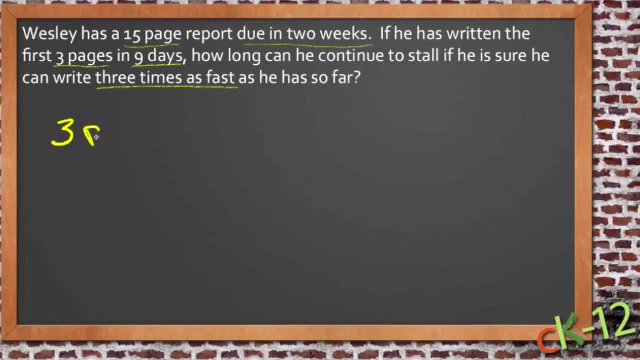 know he's written three pages in nine days. So if he's written three pages in nine days, three-ninths reduces to one-third. So so far he's been writing one-third of a page per day. So each day he writes another one-third of a page. 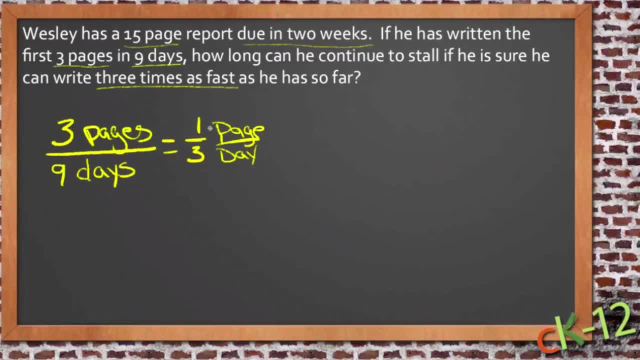 That's why it's taken him nine days to write three pages. Now, if he were to continue at that rate, he has three pages done out of his fifteen pages. so he needs twelve, Twelve more pages If he were to continue at this rate- a third of a page per day- then it takes 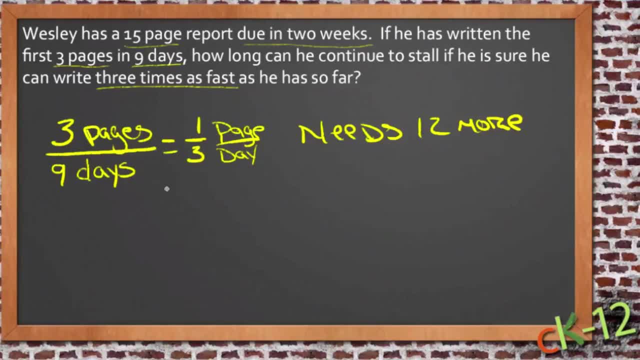 him three days to write a single page. So at this rate, three days per page, that's right. It would take him three times twelve or thirty-six more days. So obviously he's going to have to step up his pace a lot, right? So if he thinks he can actually write that, 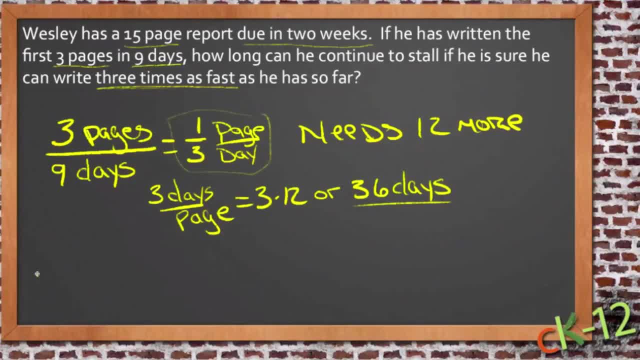 three times as fast as he had, then instead of writing at a third of a page per day, we'd have three times one-third of a page per day, which would mean that he'd write a whole page day, because our threes would cancel, right? so if he writes three times as 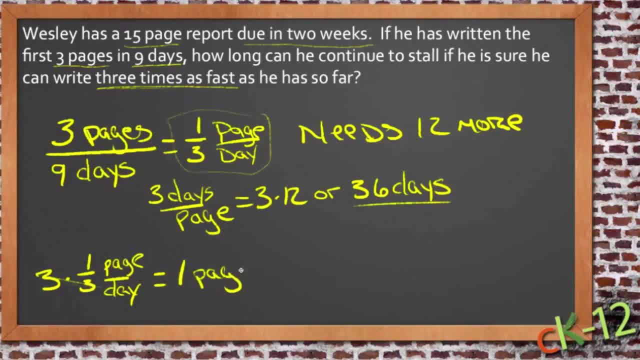 fast, as he has been, then he'll write one page per day and he needs 12 more pages. so one page per day times 12 days, the AY would be 12 more days. so if he has two weeks left, that's 14 days. then we have 14 minus 12 or two days that he can still. 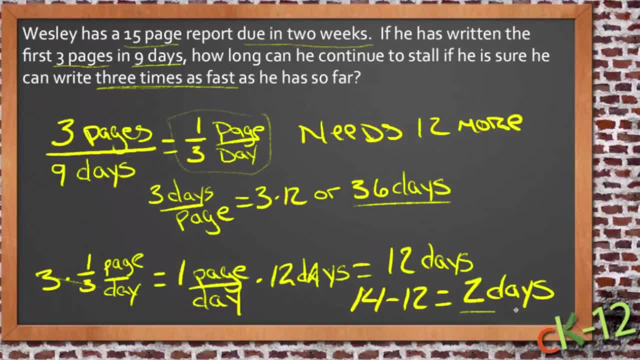 mess around and not get to work, assuming, you know, he really does think he can work three times as fast as he has been and that in two more days he's not going to be looking to see how much faster he'd have to work to stall one more day. 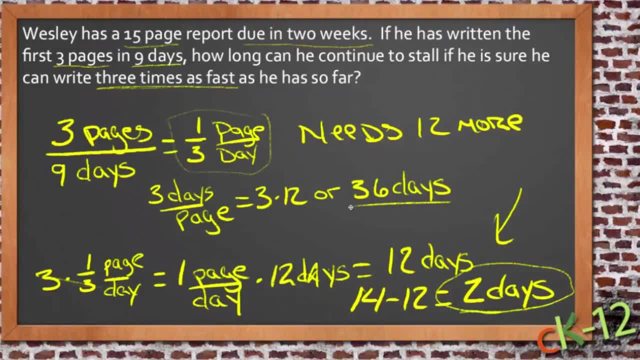 so there's, using a linear equation, really a linear process- I suppose that wasn't really a very good linear equation, but a linear process to solve a real-world problem- and what we did here was really find the rate of change, which was the slope of his information. so the slope here was 1- 3rd, 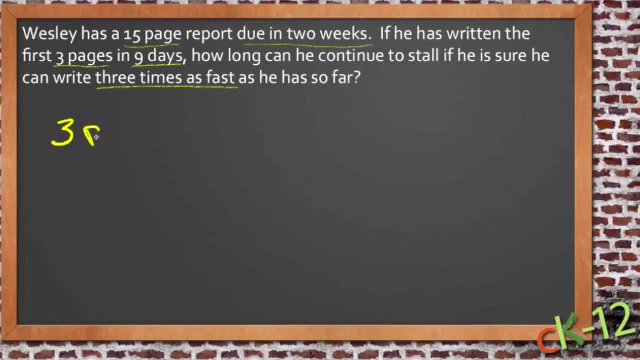 know he's written three pages in nine days. So if he's written three pages in nine days, three-ninths reduces to one-third. So so far he's been writing one-third of a page per day. So each day he writes another one-third of a page. 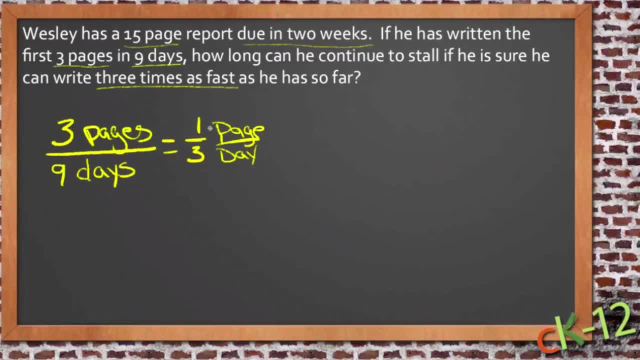 That's why it's taken him nine days to write three pages. Now, if he were to continue at that rate, he has three pages done out of his fifteen pages. so he needs twelve, Twelve more pages If he were to continue at this rate- a third of a page per day- then it takes 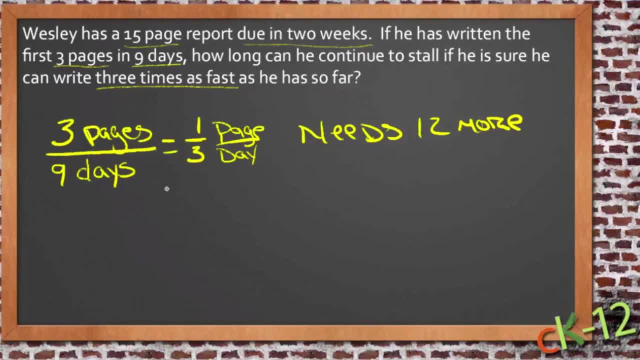 him three days to write a single page. So at this rate, three days per page, that's how long it would take. It would take him three times twelve or thirty-six more days. So obviously he's going to have to step up his pace a lot, right? So if he thinks he can actually write that three times, 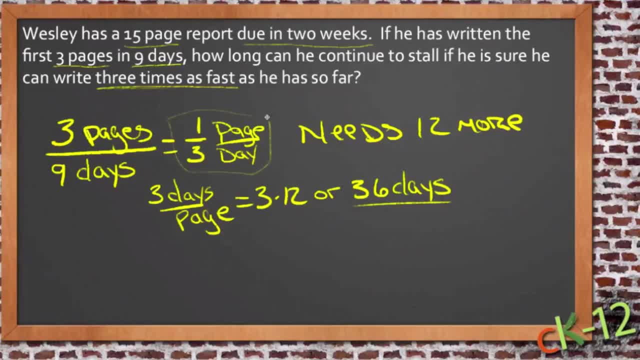 as fast as he had, then instead of writing at a third of a page per day, we'd have three times one-third of a page per day, Which would mean that he'd write a whole page per day because our 3's would cancel right. 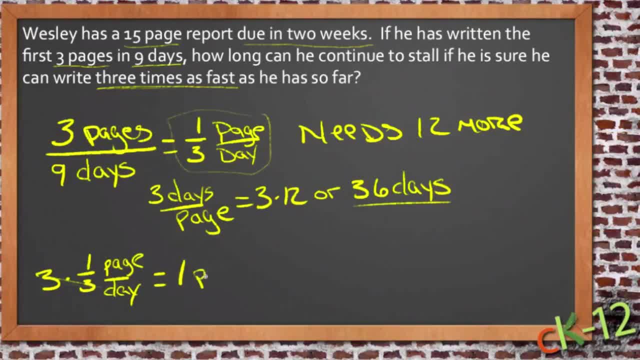 So if he writes 3 times as fast as he has been, then he'll write 1 page per day And he needs 12 more pages. so 1 page per day times 12 days, D-A-Y would be 12 more days. 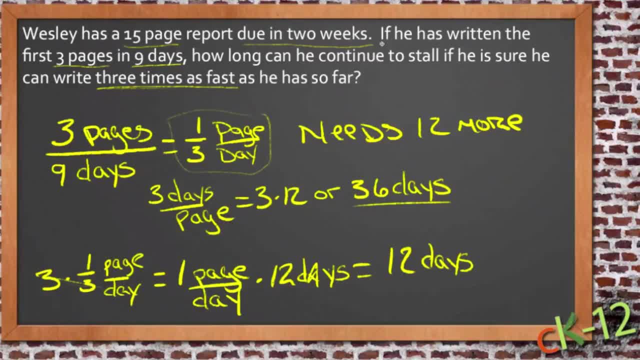 So if he has 2 weeks left, that's 14 days. Then we have 14 minus 12, or 2 days that he can still mess around and not get to work, assuming he really does think he can work 3 times as fast as he has been. 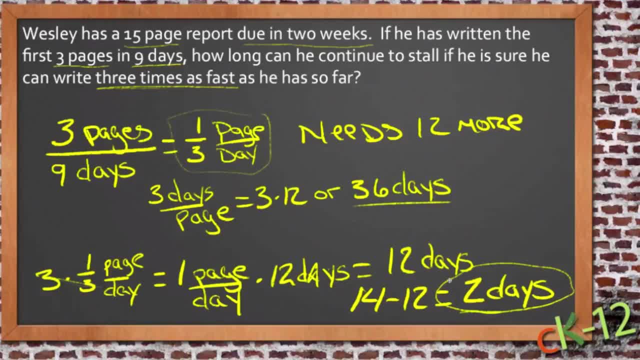 and that in 2 more days he's not going to be looking to see how much faster he'd have to work to stall 1 more day. So there's, using a linear equation, really a linear process. I suppose That wasn't really a very good linear equation. 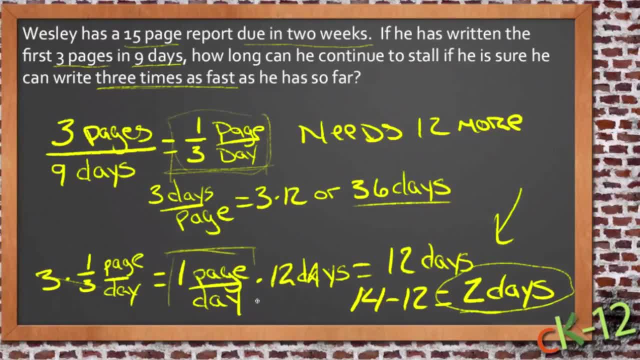 and then find the second slope of the increased rate, which was 1 over 1. then we applied those slopes to a given input, in this case a number of days, to see how many papers or how many pages he could write using the slope that we had in. 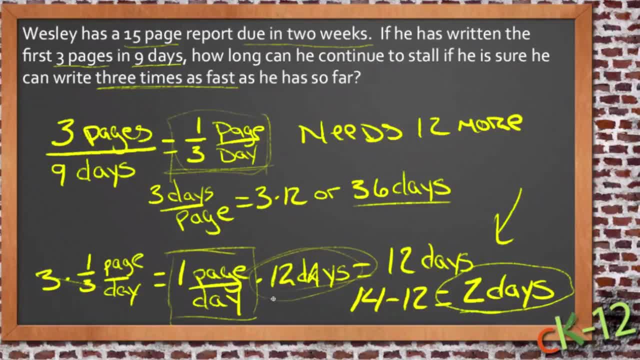 that time. so it was a linear equation. it was just sort of applied directly to the real world. so there you go. 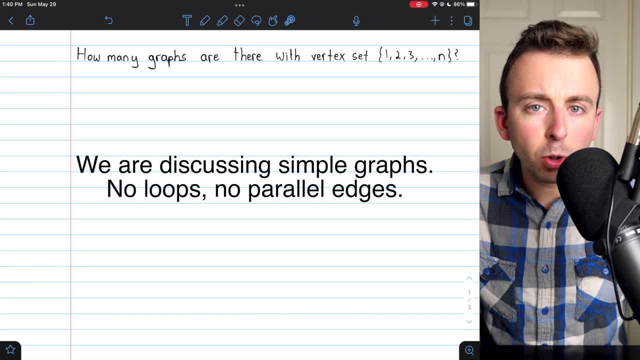 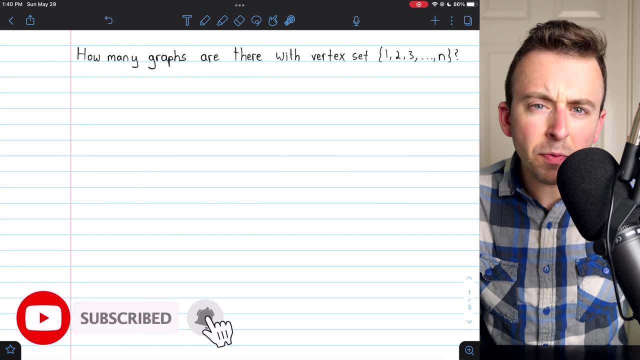 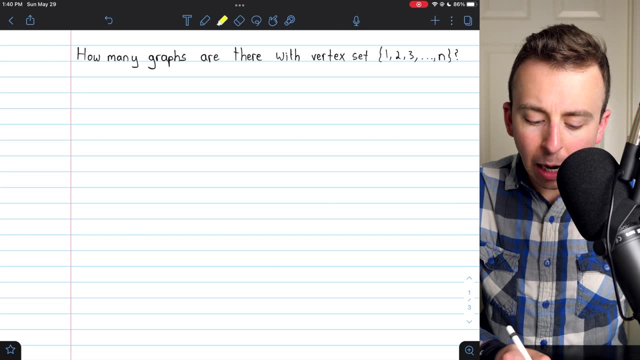 Once we start talking about graph theory, a pretty natural question emerges, which is: how many graphs are there? Well, of course, there are infinitely many graphs. but more specifically, how many graphs are there on n vertices for a fixed n? Or, put another way, how many graphs 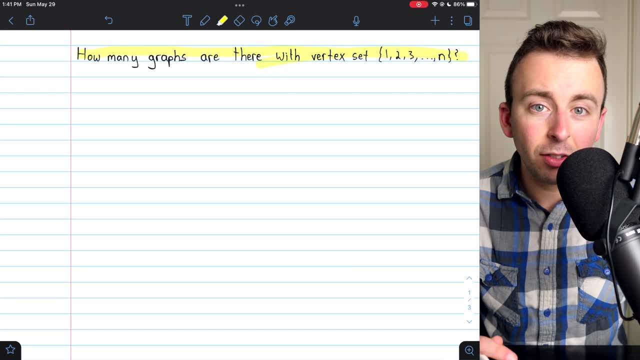 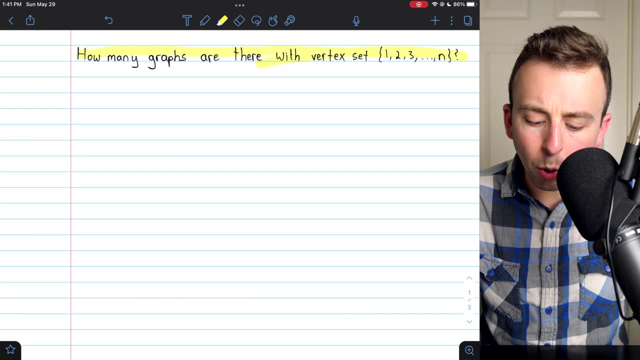 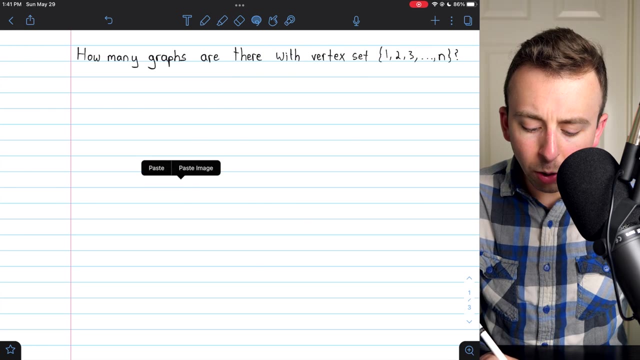 are there with vertex set 1 through n. So 1 through n are the labels of the vertices. It turns out this is actually a pretty simple question to answer, as long as we're not too picky about how we're counting graphs. So in this video we'll be counting labeled graphs. 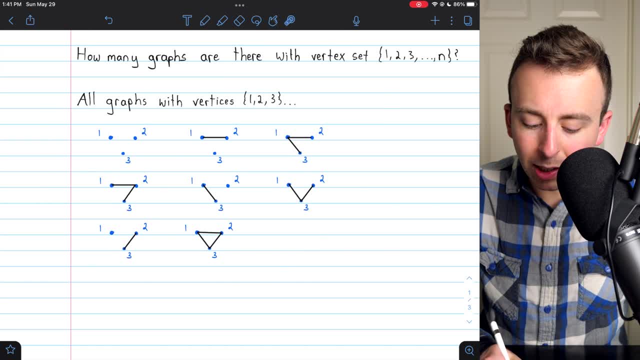 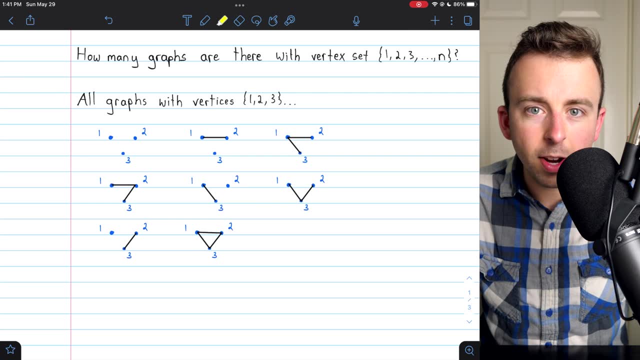 By that I mean, for example, here are all of the graphs with vertices 1,, 2, and 3.. So for our purposes, the answer to the question how many graphs are there with vertex set 1,, 2,? 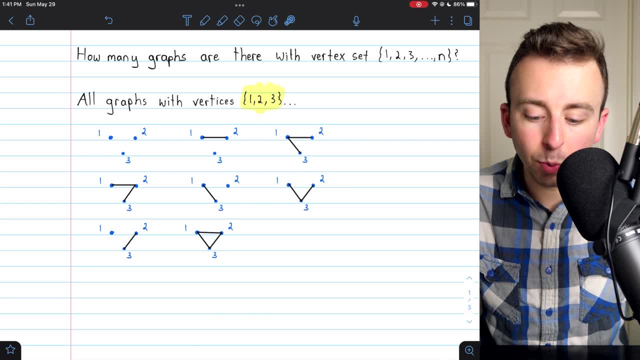 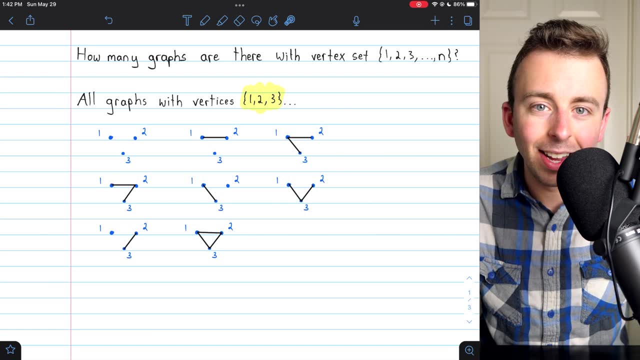 3, would be 8.. There were 8 different graphs with that vertex set and here they are here. Of course, if we called the vertices A, B, C or X, Y, Z, that would not change the question very much. But here are the 8 different graphs.